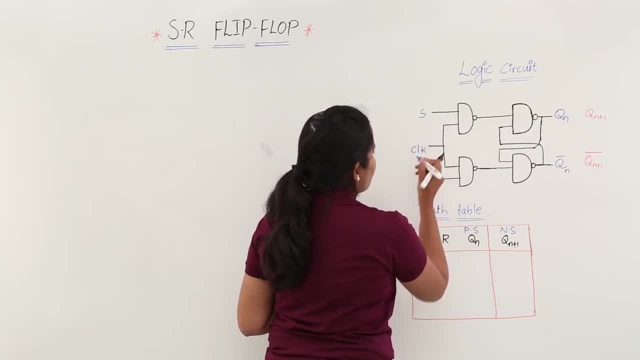 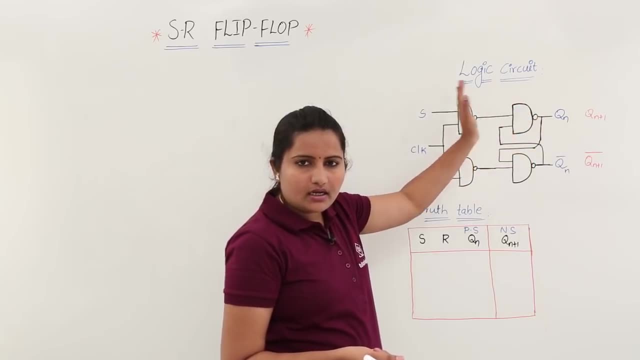 input. you can say this is clack input for SR flip flop Previously for latches. we are having this as latch, So we are ah giving some clack put, ah clack pulse circuit. So this is going to become as flip flop that. 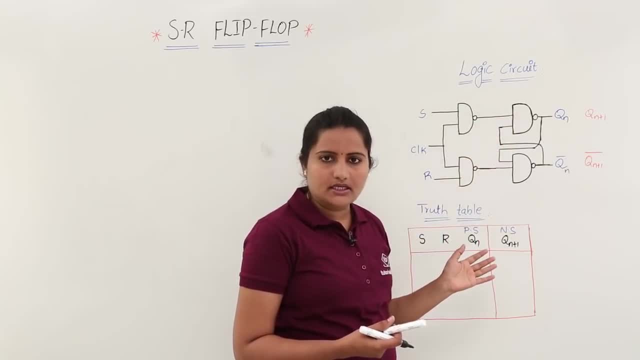 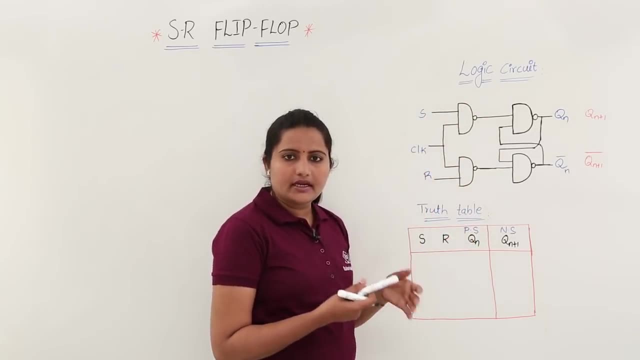 is it So up to here? this is a ah flip, actually a latch, and by giving some clack pulse, like this circuitry, by just adding this circuitry, we are, ah, maintaining this as flip flop. So here Now, when you saw this. third, 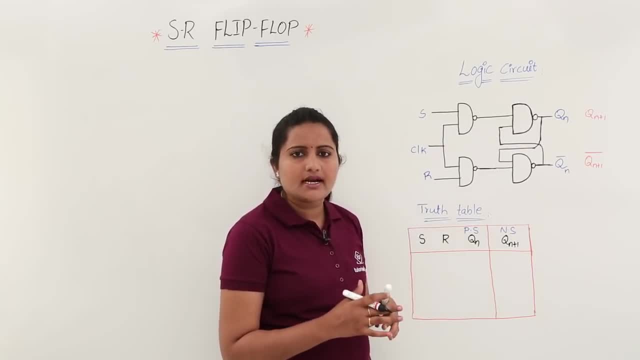 type of structure everyone are going to misunderstand, like qn and qn bar, are outputs, our outputs, required outputs? yes, those are outputs, but not our required outputs. those are just present state of that flip-flop or latch present. state is nothing, but that is, ah. input feedback. 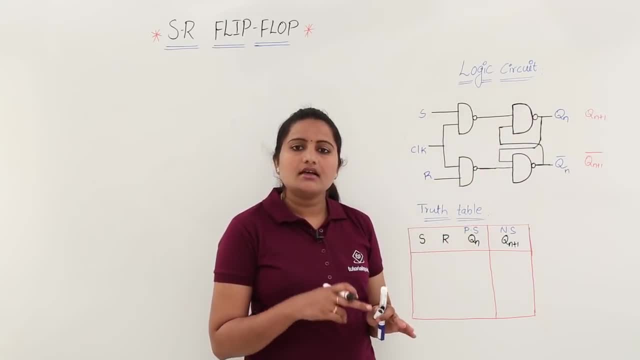 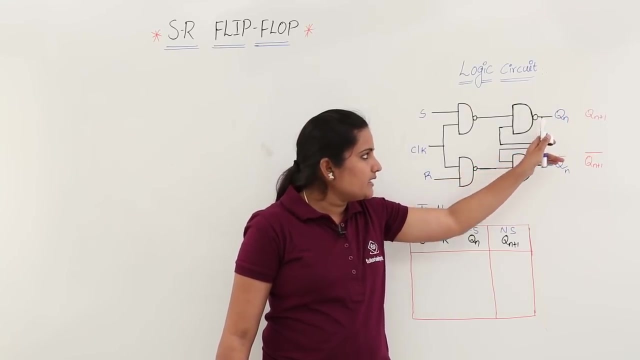 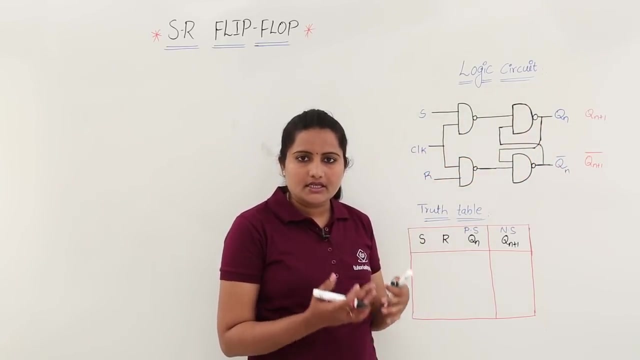 input. for our circuit that means present state is nothing but output. of output came from past inputs, so that is not our required input. always you need to check for next state. next state is nothing but by taking the reference of this present state and my present inputs. so whatever we are getting as 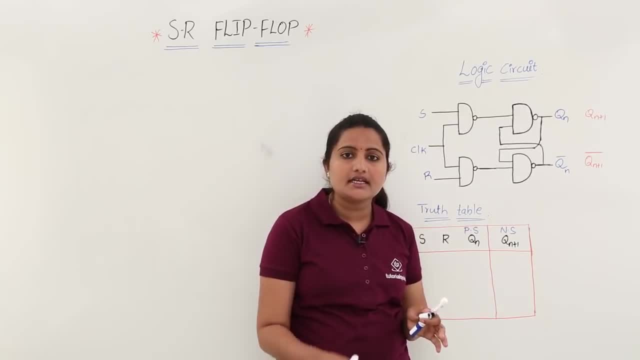 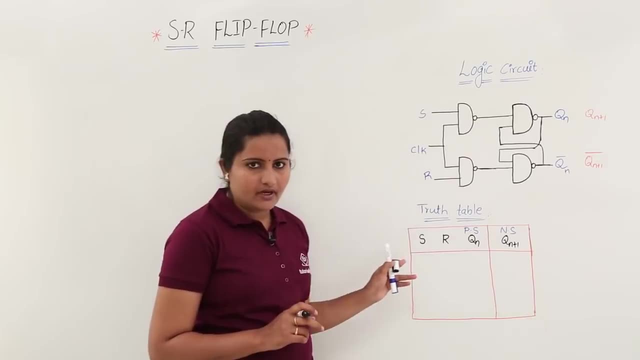 output that is called as next state. that next state is our required output for any sequential circuit. so now i am going to get my functionality by using truth table. i want to represent my functionality, so my inputs are ah, s and r set. reset inputs i am giving, and here ah, qn is present state. this is: 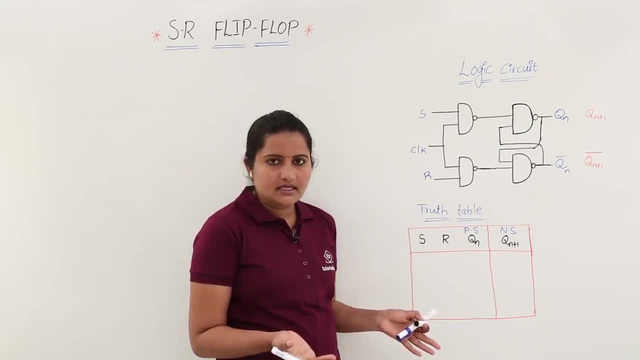 also taken as reference, but we do not know that present state. so because anyone given you a circuit like sr flip-flop or anything, we do not know the present state, in which state that is in, we do not know. so just we need to give input sequence. that means s and r values. you need to. 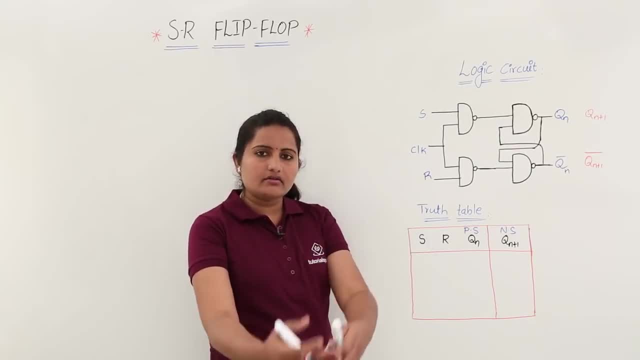 give either 0, 1 or 1, 0, like that. you need to give input sequence that means s and r values. you need to give input sequence that means s and r values. you need to give input sequence that means s and r values. like that it is going to give next state, that next state we need to define here. so here my sr. 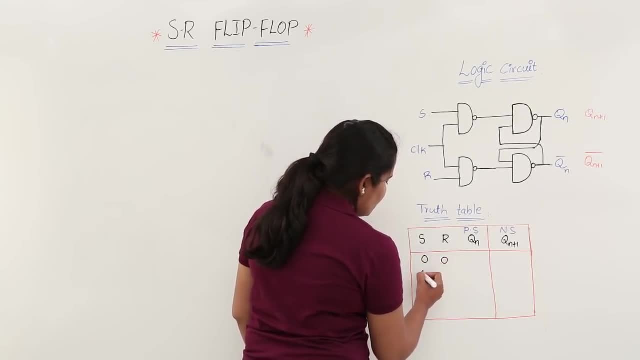 may be either 0, 0, 0, 1 and 1, 0 and 1: 1. we do not know this present state, but we are taking as reference to get my next state, that next rate i am going to define here. so first ah, combination i am taking. when s is equal to zero, r is equal to zero, what may will be the state, moderate phase, positive values. the p through negative phase, a over t, if negative phase. the structure of the creatinine, professor Bin: 0 and b. the current phase format. so the current phase, simplifying normalization. 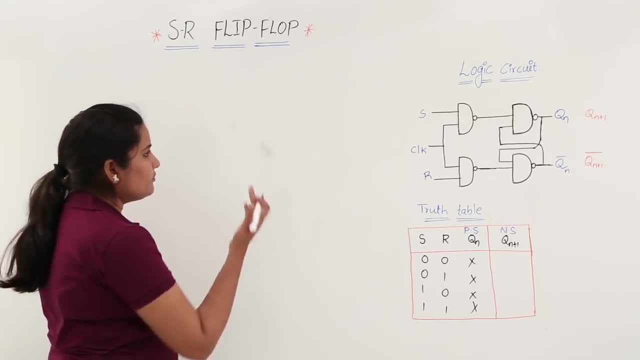 of the Plaza algebra. so this is our current phase, but it means we can use similar fractions, that isacial to prime and waiting that is, thising upพ loved our peak with this periodicELL equal to 0,, what may be my next state of machine. So here I am considering my first example. 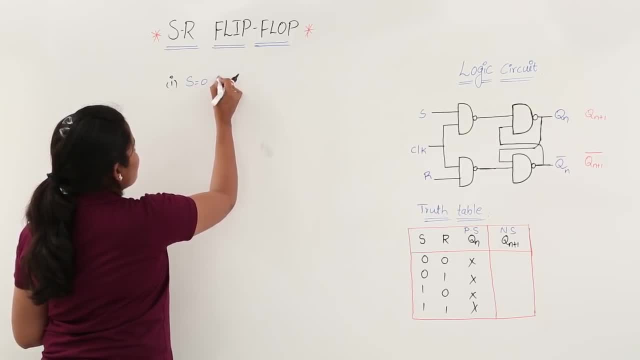 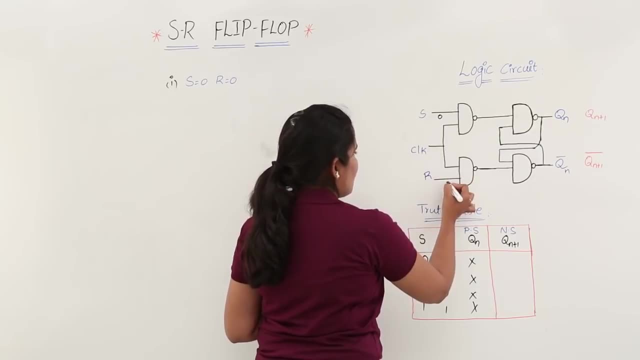 that means first combination of S, R, S equal to 0, R equal to 0. So in this condition, in this case, if I given S equal to 0, R equal to 0 and the clack pulse, here I am taking. 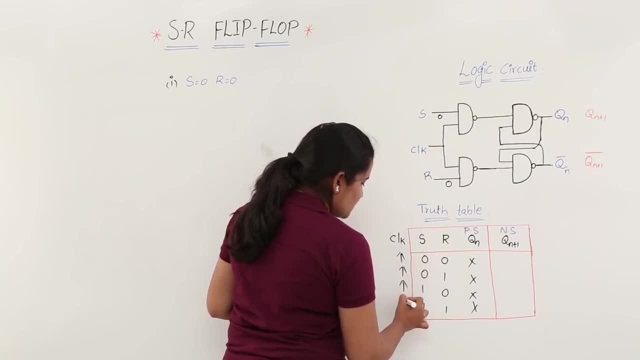 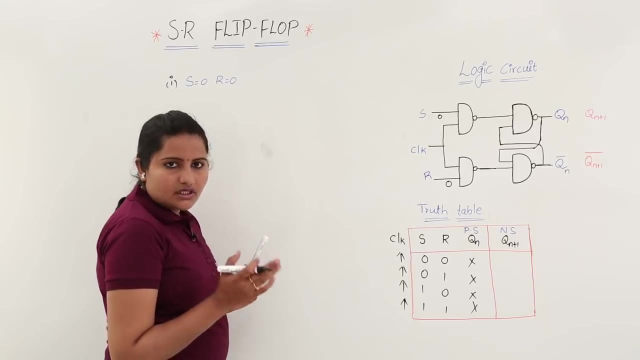 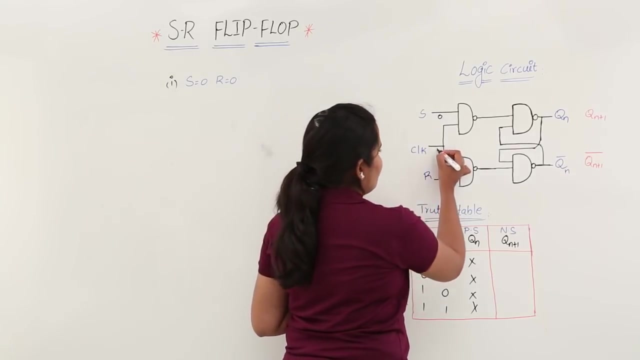 clack, pulse is on. clack pulse is on means so here clack is equivalent to 1.. So here, when clack equal to 0, I will give you after completing this, when clack is equal to 1, what you are getting. So always clack need to be 1 to trigger that flip flop. So here, 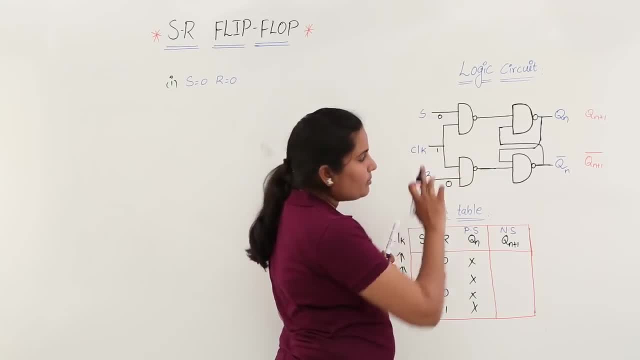 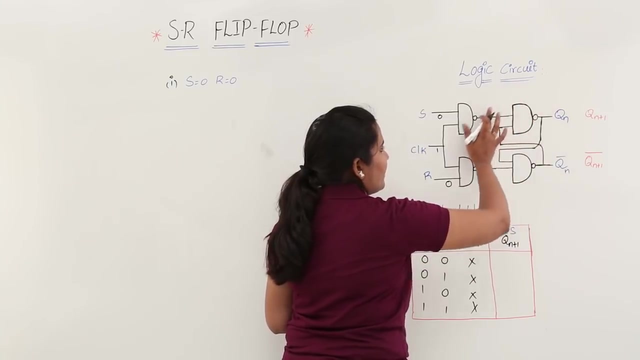 0 into 1, you are getting 0 bar. you are getting here into 1 bar. you are getting 1 here. Again, here also, 0 into 1 whole bar. you are getting 1 here. So you just keep in mind when, when, when you got at the output of SR, latch what. 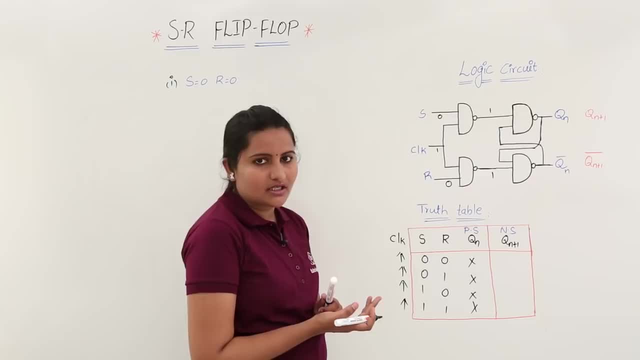 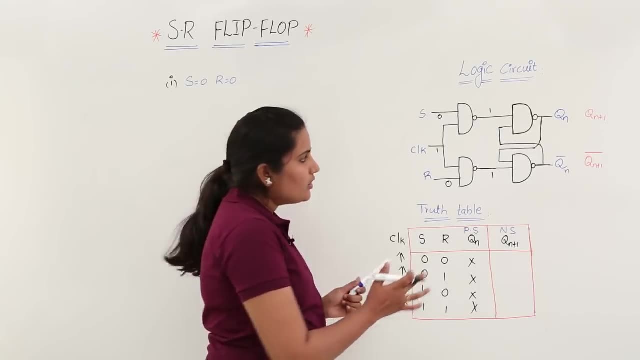 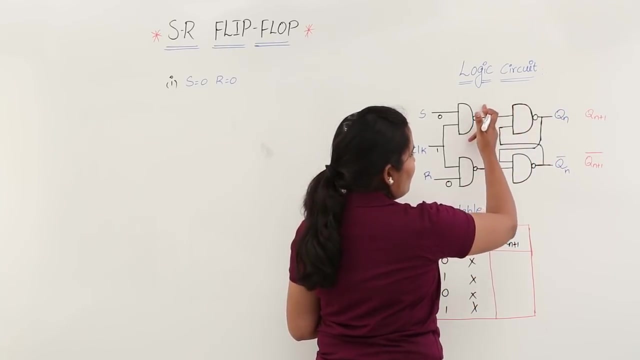 you are getting. Obviously you are getting no change condition right For SR latch by using NAND gates. you can see previous class also When 1: 1 condition you given for this latch circuit, you are getting no change condition. You can observe here: 1 into q n bar whole. 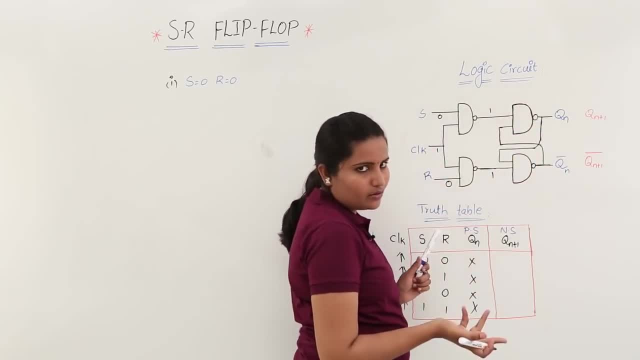 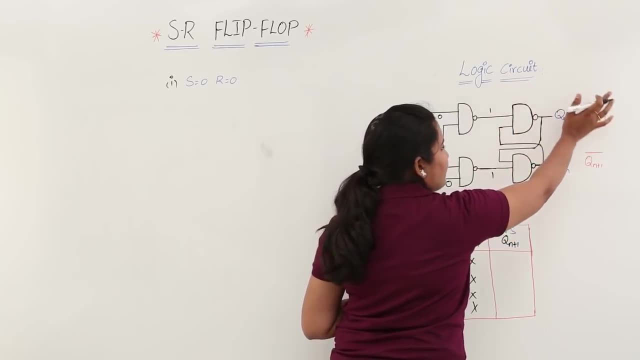 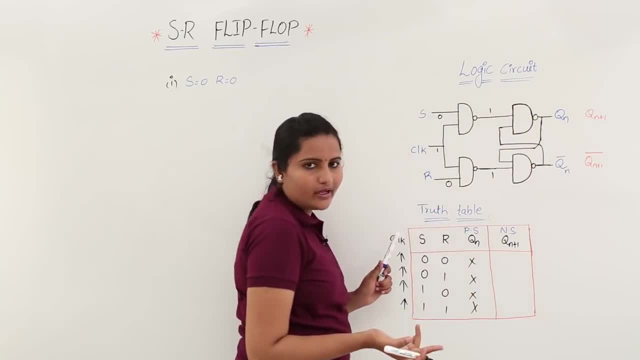 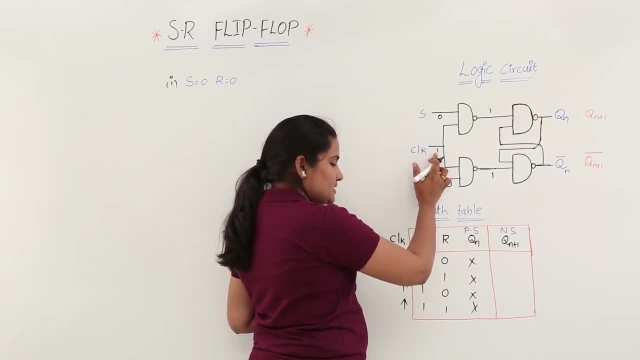 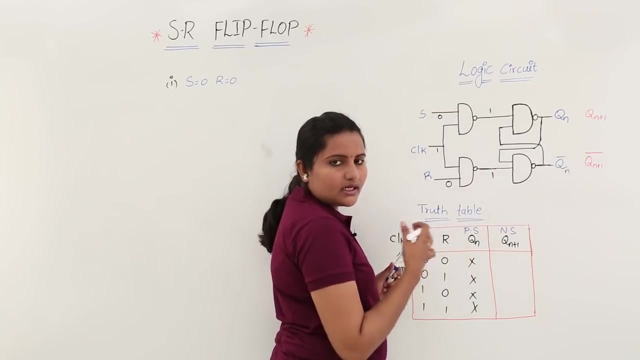 n bar into 1. whole bar is equivalent to q n. only that means no change state. So here you are getting when you, when your clack pulse is 1 and when you are providing SR equivalent to 0, 0.. So here you are getting 1, 1.. So that will provide no change, condition that: 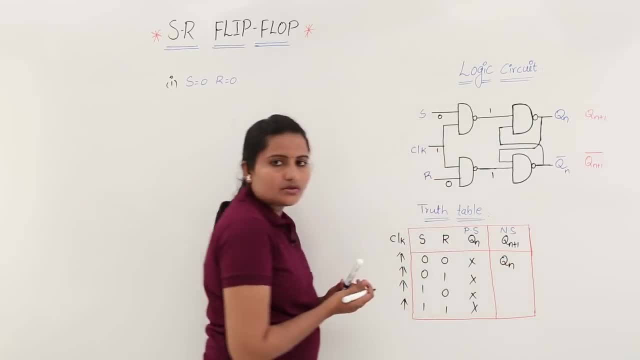 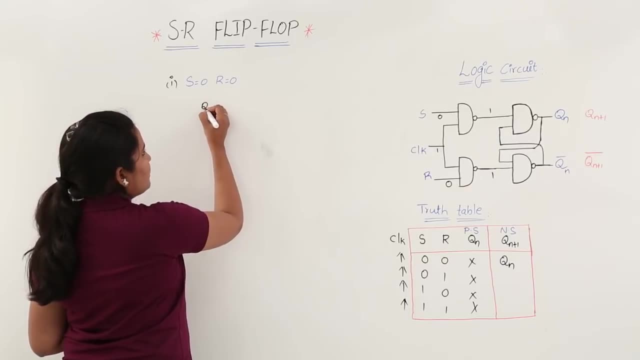 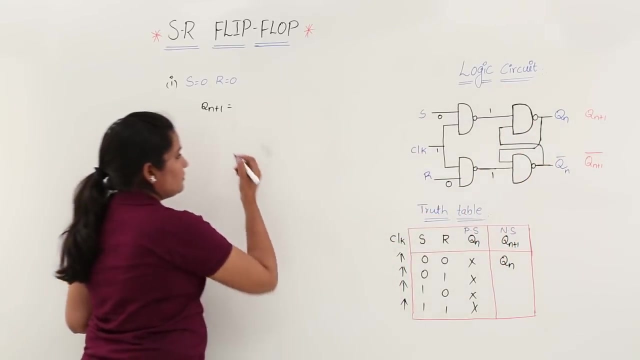 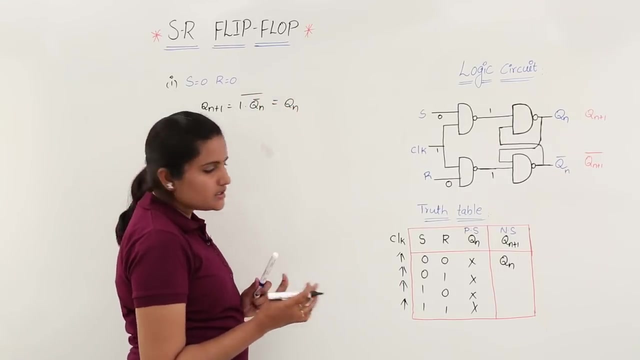 means q n here. So that means here I am taking, So here I am taking q n. q n plus 1 is equivalent to: So this thing I am writing, So I am just processing. So 1 into q n bar, whole bar, you are getting q n. This is my first condition. 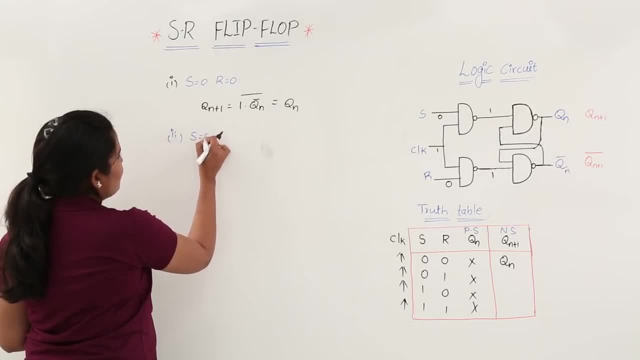 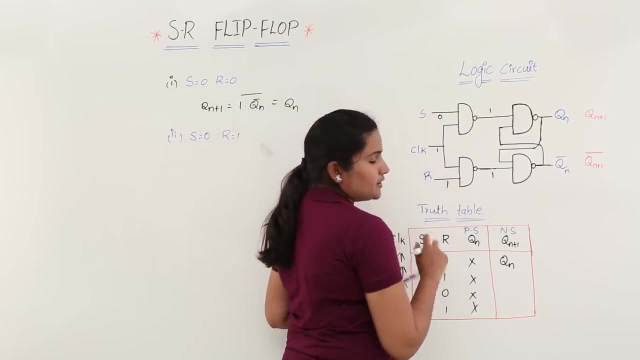 My second condition is S equal to 0 and R is equivalent to 1.. So if you given S equivalent to 0 and R is equivalent to 1, then 0 into 1. whole bar again here: 1 is there, but here. 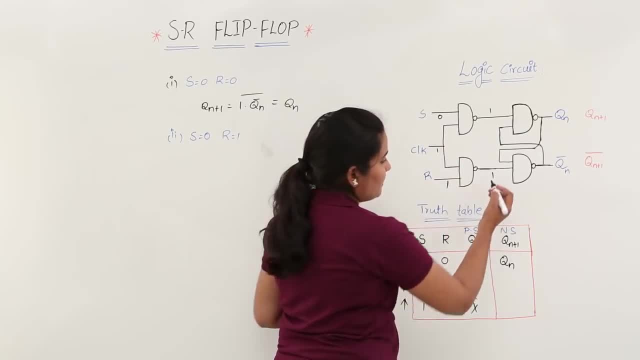 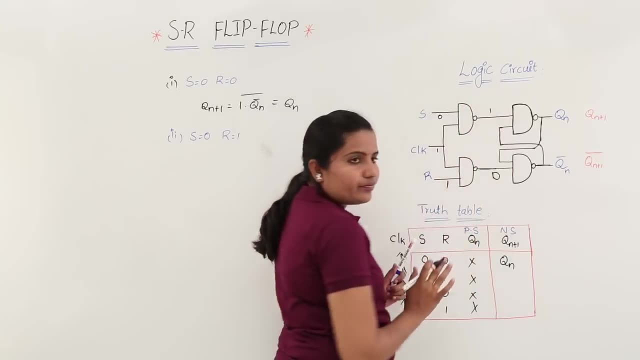 1 into 1 whole bar. 1 bar will come. that means here you will get 0 in place of 1.. So now, when you got 1, 0, then your flip, your flip flop, is going to reset. see here. So this: 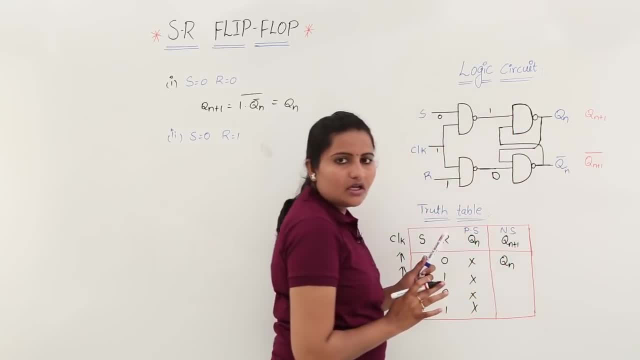 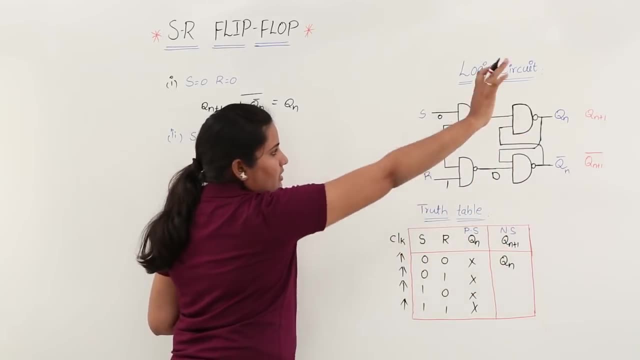 is a latch circuit. for a latch circuit, if you given 1, 0. Your latch is going to reset, So you just check here. So, for example, so I am taking normal port for q n plus 1, if I want to write, then 1 into q n bar, whole bar, 1 into q n bar. 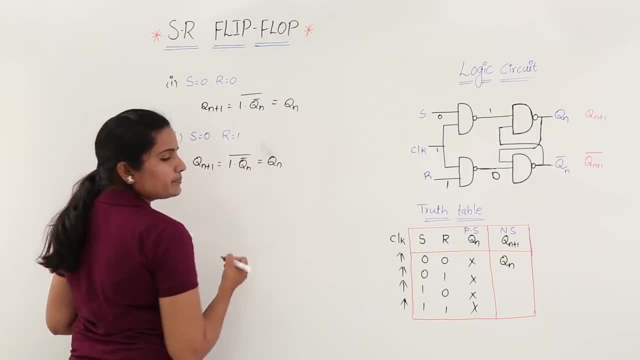 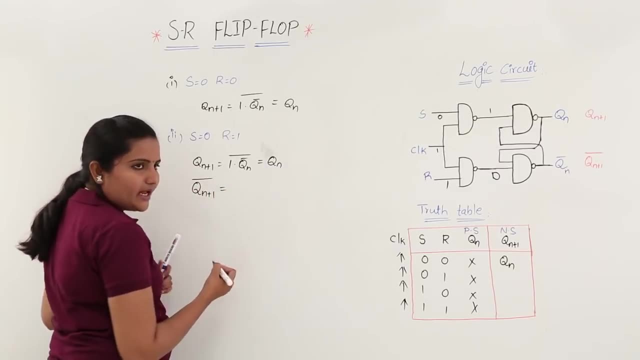 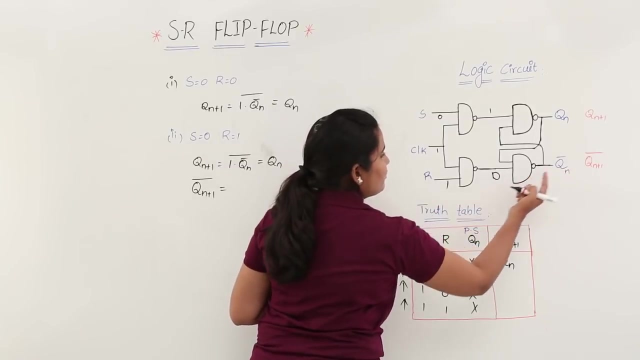 whole bar. So this is equivalent to q n you are getting. You did not got any value, So you you just checking in a complementary port. if you are getting value, then you can even imply for that normal port. So I am checking q n plus 1 bar port. that that means this port. 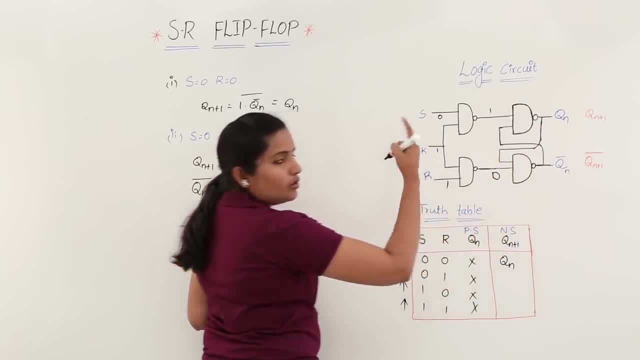 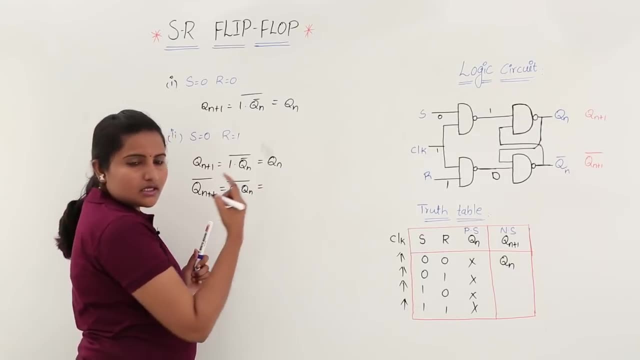 output. So here, 0 into qn whole bar, you are getting 0 into qn whole bar. this is equivalent to 0 into anything. 0, 0 bar means 1.. If qn plus 1 bar is equivalent to 1, then definitely qn plus 1 value maybe complement of this That. means this may be is equivalent to 0.. Now we are going to dear one more function to run it from, maybe白iquement value. It is going to be a contains problem, like pen cylinder. it is going to be going to onde by the same formula. This is the firing不錯, so that the 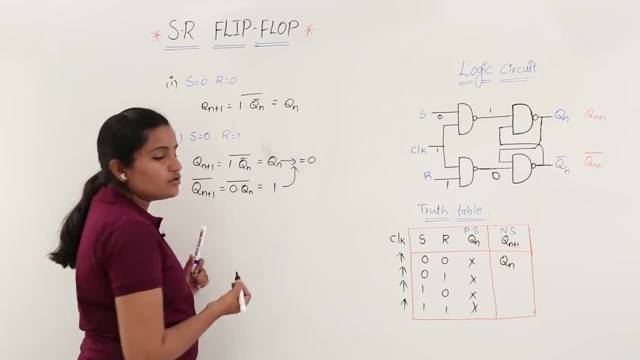 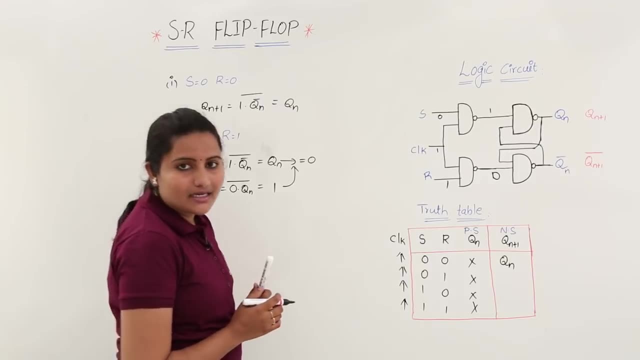 output will be the same. So if violet is equal, then when we mean theietet, that to yellow is equal to 1.. This, with reference of this, this value may be equivalent to 0.. So, finally, in case of S equal to 0 or equal to 1, you are getting reset condition of SR flip-flop, So 0, so 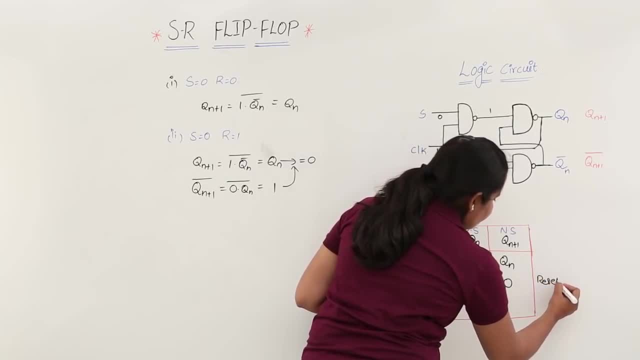 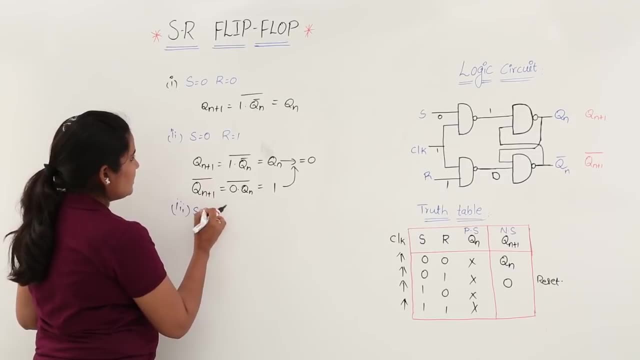 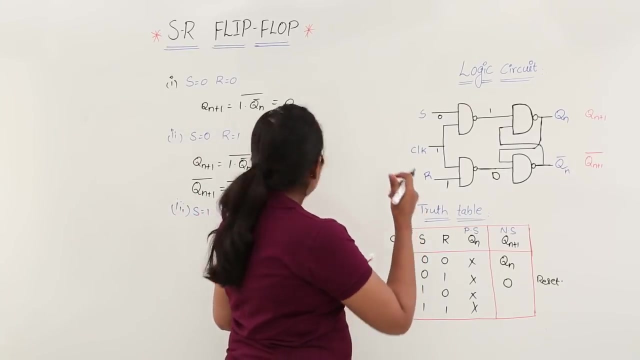 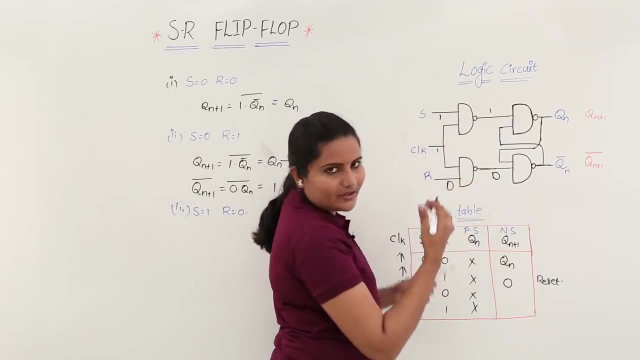 this is called as reset condition. So now in third case- I am taking third case of SR flip-flop- S equal to 1 or equal to 0. In this case your SR flip-flop is going to set C here. So if S is equivalent to 1 and R equivalent to 0, what is going to happen? Reverse of. 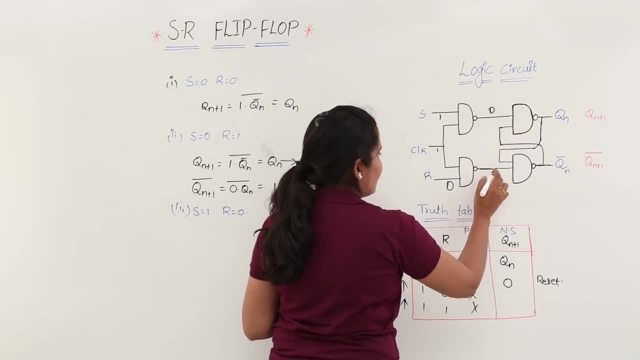 this. just you are getting 0 here and you are getting 1 here, So it is nothing, but you are getting complement of output also. So see here. so when you give an 1: 0, 1 into 1 whole bar 0 and 1 into 1 whole bar 0. So when you give an 1- 0, 1 into 1 whole bar 0. 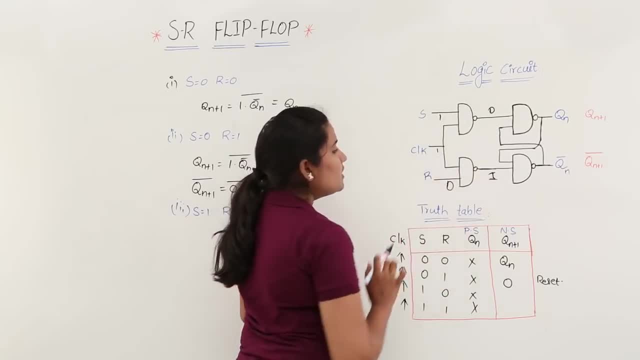 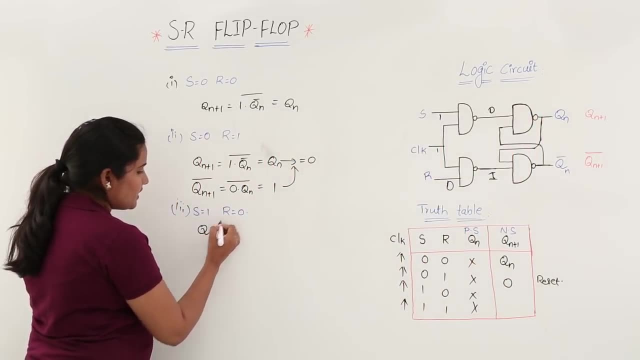 1 into 0 whole bar. So you are getting 1 here. So now, if you given 0, 1 here, what is going to happen? I am just writing here: when s equal to 1, r equal to 0, your q n plus 1 is equivalent to. 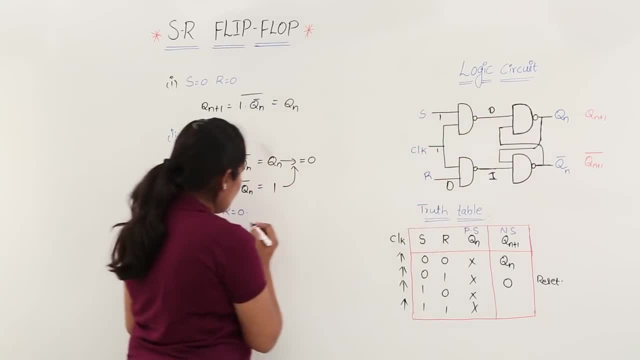 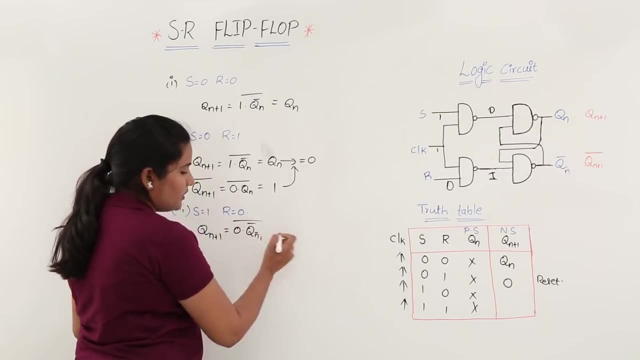 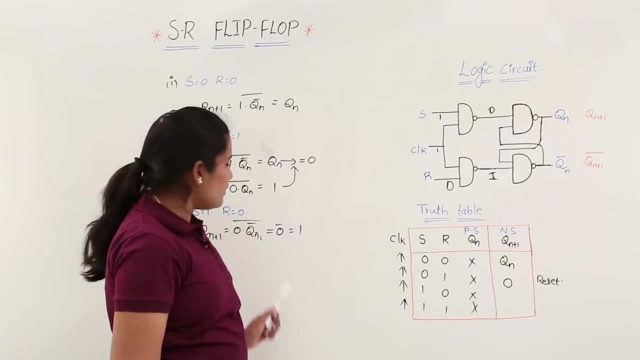 So I am taking this for: 0 into q n bar, 0 into q n bar, q q n bar whole bar, 0 into q n bar whole bar. So this is equivalent to 0 into anything. 0, 0 bar is equivalent to 1.. You got the value of. 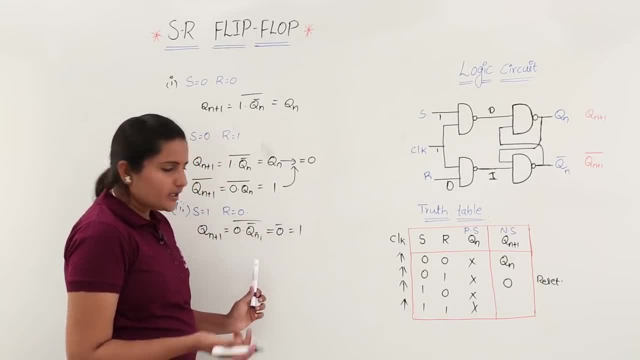 q n plus 1, then no need to go for q n plus 1, q n plus 1 complement. Why? Because if you know q n plus 1, then only you can say q n plus 1, whole bar equivalent to 0. If you got like this, that means 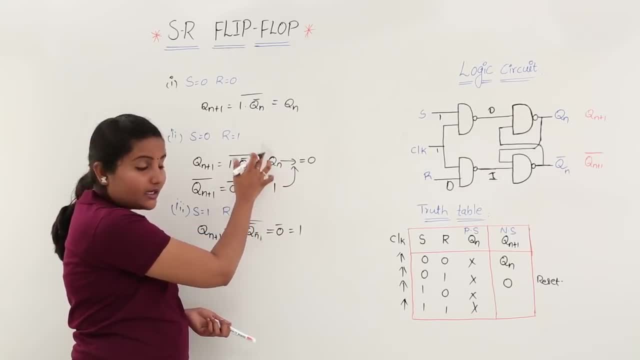 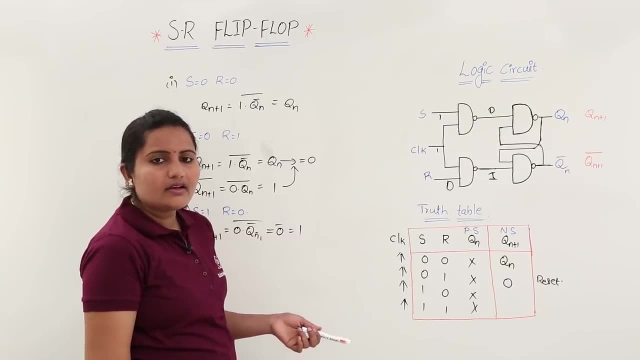 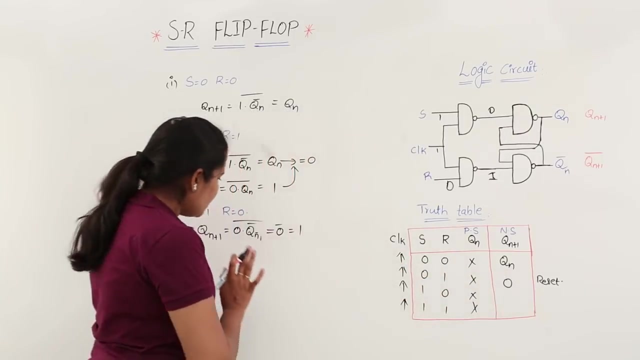 if you are not getting value in normal port, then you need to check the complement port for any value. sometimes For complement port also, no value will come to take as reference. Then we cannot do anything. you just write like this only: So here I am writing So 1 here. So this is called as. 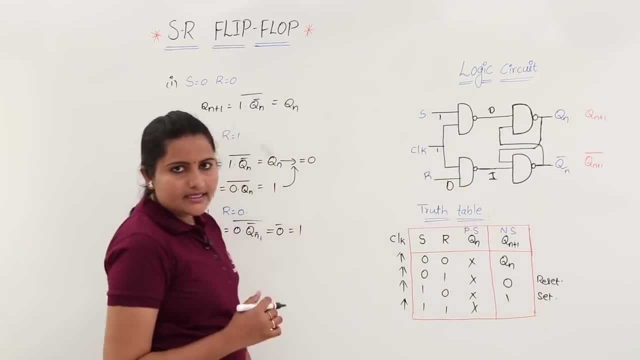 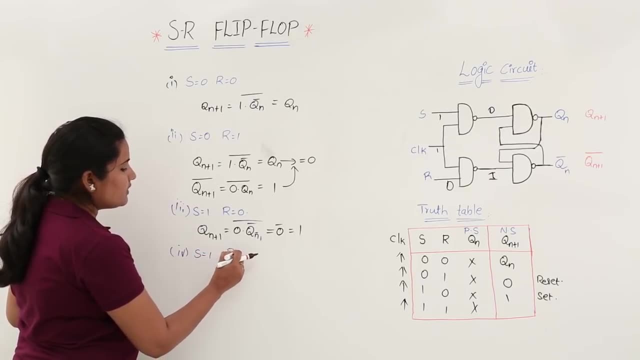 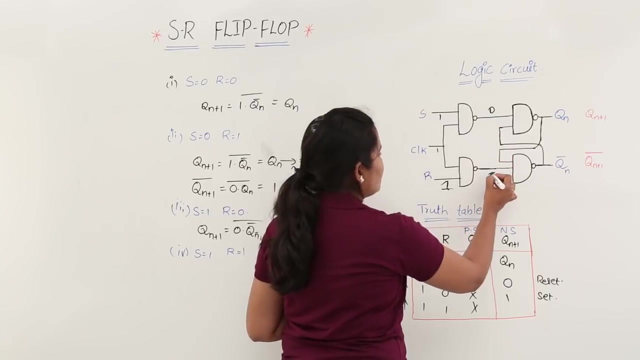 set condition of s? r flip flop. Finally, we are having fourth condition, that is, s equivalent to 1 and r is equivalent to 1.. So when you given s equivalent to 1 and r is equivalent to 1, 1 in both ports. 1 into 1 whole bar, you are getting 0,. 1 into 1 whole bar, you are getting 0. 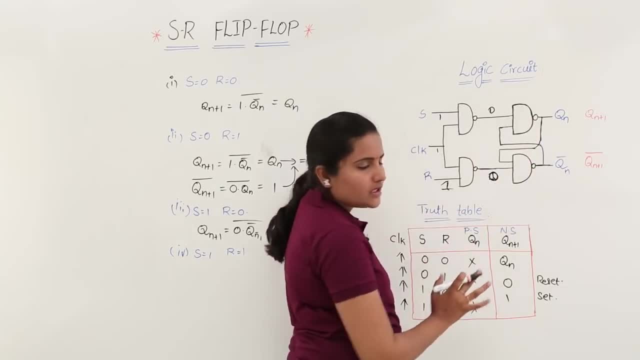 If you given 0, 0 for this latch, So this is up to here, this is a latch right. So, for example, if you are giving 0, 0 for this latch, then your condition is going to be undetermined, because not, we cannot determine this state. because 0 into anything bar, you are getting 1 and here also 0 into. 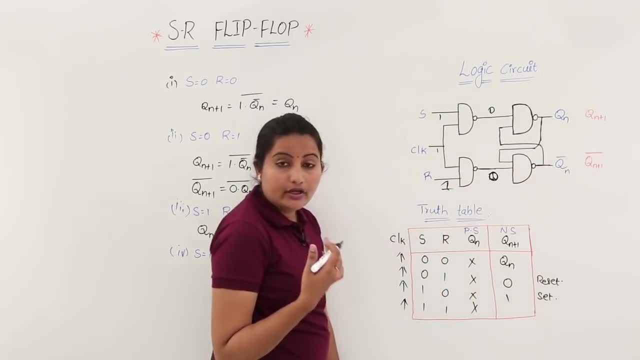 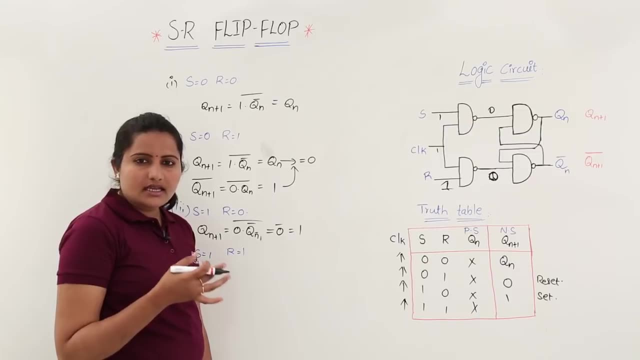 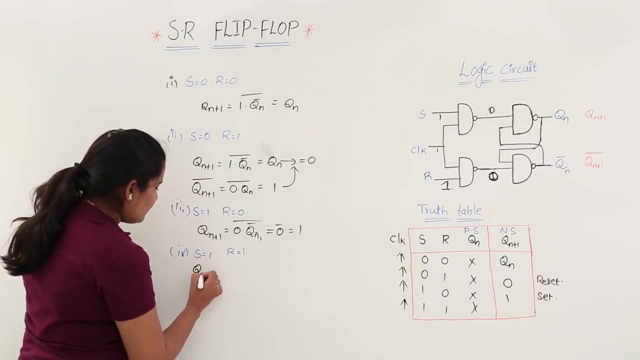 anything bar, you are getting 1.. For q n plus 1 and q n plus 1 bar, you are getting same output. that that means if a variable is getting same output for its complement and for that means that is not determined. So in this case q n plus 1 is equaling to 0 into q n bar, whole bar, you are. 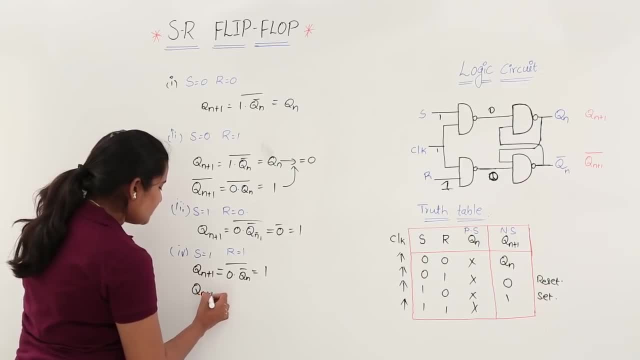 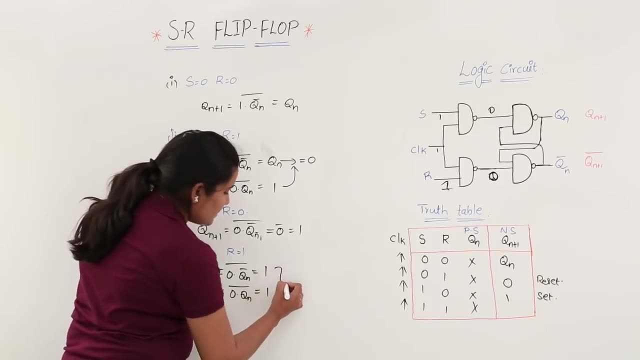 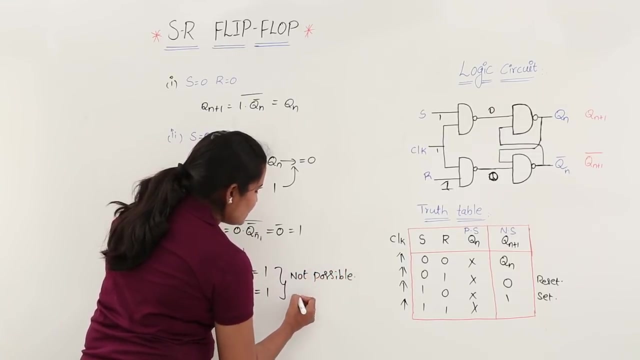 getting. here also you are getting 1.. So q n plus 1 whole bar, also 0 into q n whole bar. you are getting. That means here also you are getting 1.. This condition is not possible. This is not possible. So it can be treated as indeterminate state. So I am just representing like id.